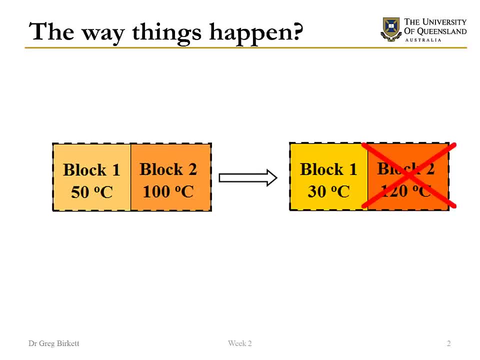 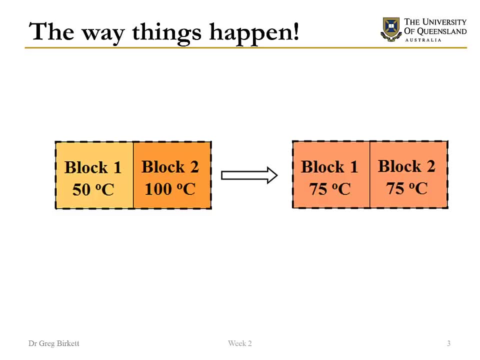 been alive, for you would know that, of course, that doesn't happen, That what would actually happen if we left these two blocks in contact with each other and they didn't lose any heat or anything to the surroundings, is that eventually you'd end up with two blocks at exactly the same temperature and according to the first. 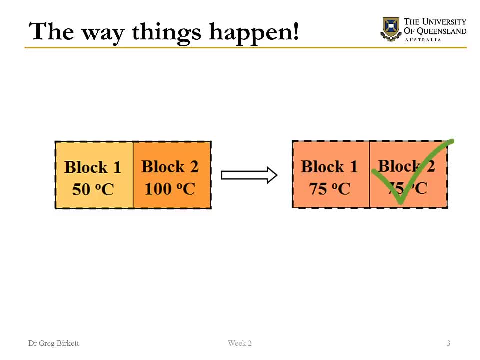 law that temperature would be 75 degrees Celsius, So this is something that we would clearly observe in real life. So what's driving this process, and can we quantify the fact that this process would happen and the process on the previous slide wouldn't? And so we've got lots of examples of where 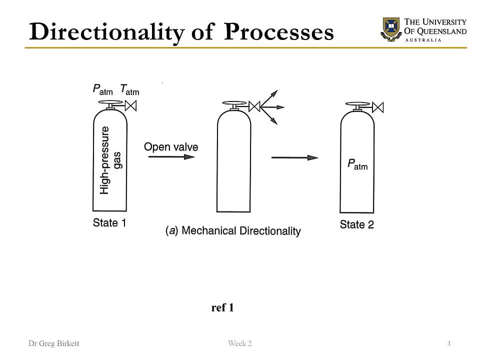 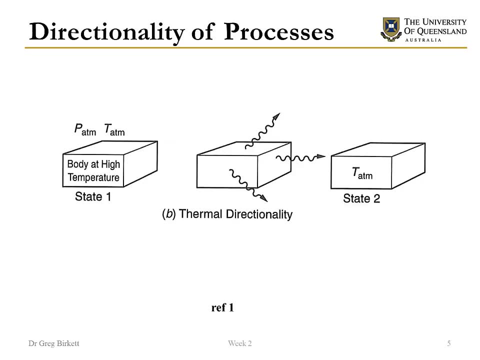 this happens. So if we opened up a gas cylinder, of course the gas would escape, never the reverse. If we had something hot and we left it sitting in a room, the the heat would escape and you'd end up with your block or whatever it is ending. 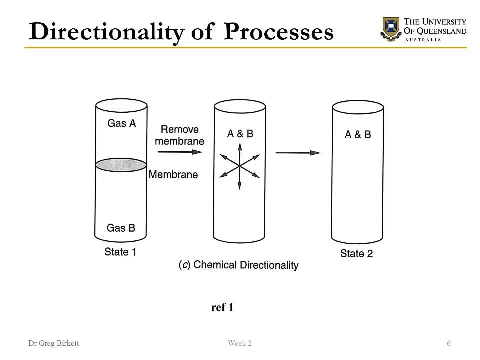 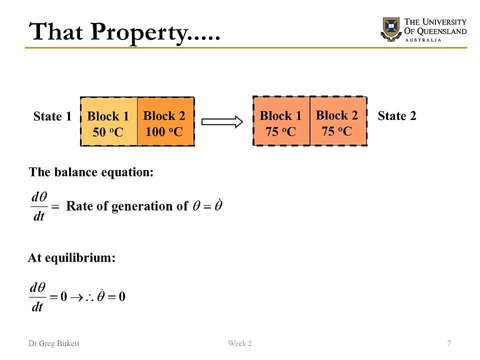 up at room temperature. Or if I had two gases separated by a membrane and I removed the membrane, the two gases would mix. All these things are sure to happen. So we must be able to quantify the fact that these things are certain to happen and not the reverse. So if we go back to our two block example, then what? 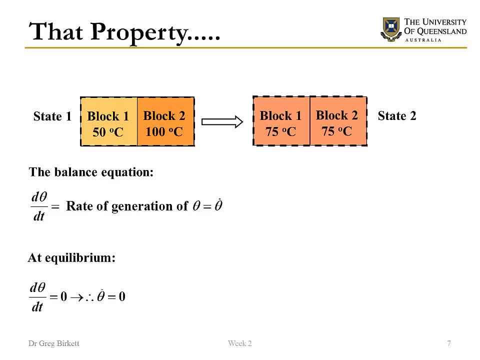 we need is: we need a balance equation that changes with time. So when we're going from this condition on the left, where we've got two different temperatures, to the condition on the right, then something has to change within this closed system with time. So this: 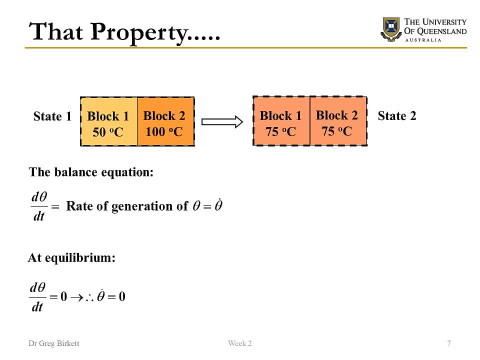 can't be a conserved quantity like mass or energy. It has to have a generation term. And then the second condition that we can put on this by looking at this is that eventually, at some point now when both blocks are 75 degrees Celsius, we'll 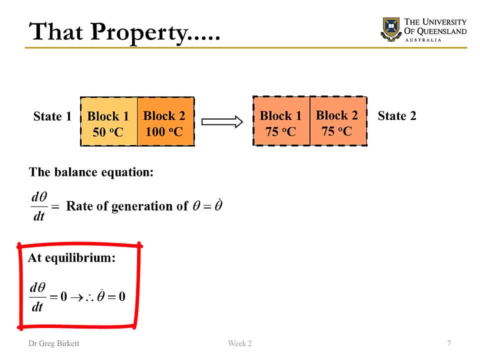 reach equilibrium. Nothing changes after this at all. So, even though there's a must be, some sort of generation term for us to change from the left to the right, when we do get to the right, then we reach an equilibrium state. So these are. 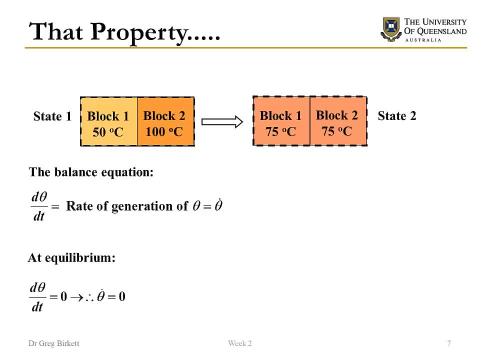 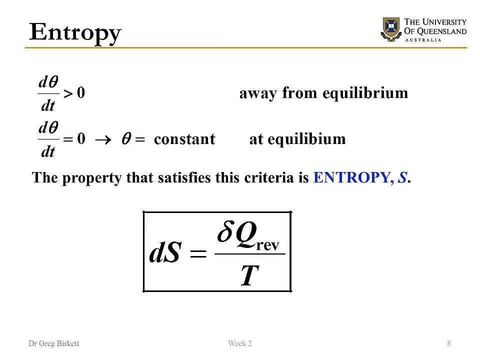 the properties that have to be met if we're going to quantify what's going on in this system. So the property that does that for us is entropy. So, away from equilibrium, we have a change in the entropy not equal to zero or greater than zero, and at 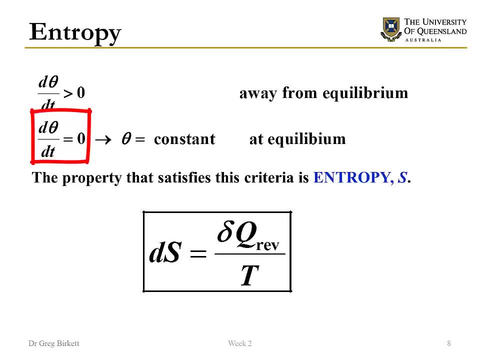 equilibrium, the change in it is equal to zero. Now the conditions of entropy or the definition of entropy. that satisfies this is this definition here: that the entropy, or an incremental change in entropy, is an incremental change in the heat added to the system divided by temperature. This is the definition of entropy. 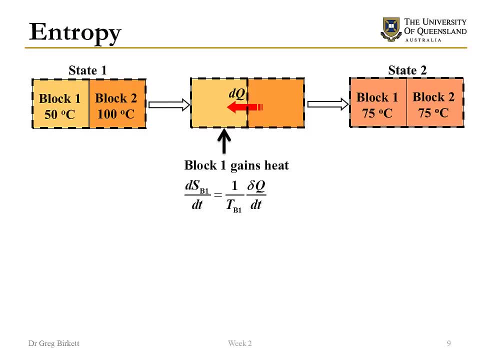 Now, if we go back to having a look at our block problem, then, and if I look at the process and going from state 1 to state 2, then heat has to be transferred from block 2 to block 1.. So block 1 gains a little bit of heat and so 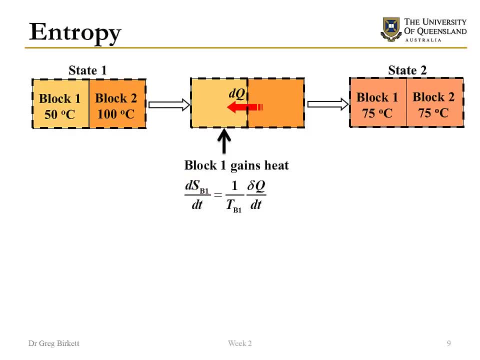 therefore it gains a little bit of entropy. Block 2 has to lose a little bit of heat and therefore it loses a little bit of entropy. Now, as per the definition, I'm dividing by this temperature term on the right hand side here. Now, if I add: 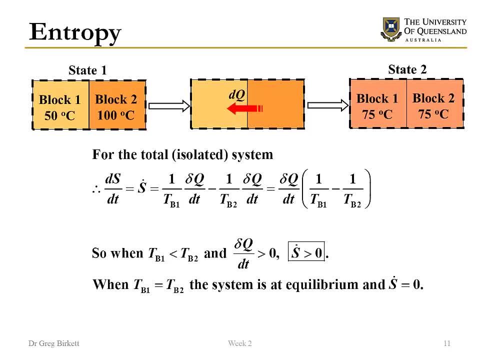 those two things together, so what's happening in block 1 and what's happening in block 2.. So for the isolated system as a whole then the change in entropy with time is equal to the generation of entropy. okay, because nothing's going in, nothing's coming out of my isolated 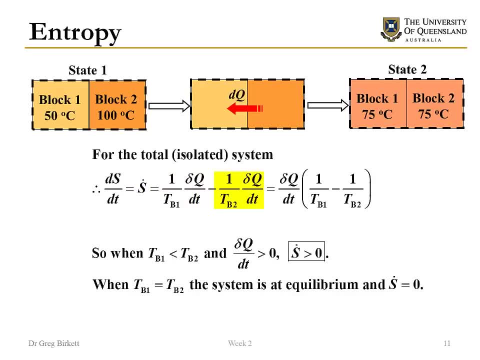 system, and I'm just adding up those two terms that we had on the previous couple of slides, and so what I see is is that when the temperature of block 1 is smaller than the temperature of block 2, then my decoder T term has to be greater. 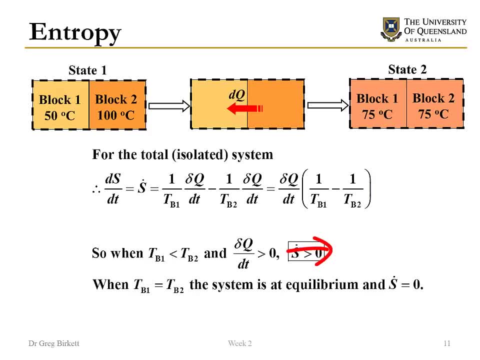 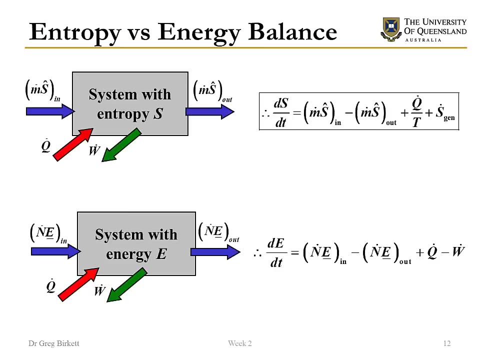 than 0 and therefore my entropy generation term is greater than zero. And it's only when my two blocks are at the same temperature that my system's at equilibrium and my entropy generation is zero. So, now that I've established the fact that there is an entropy generation term and it's a real, 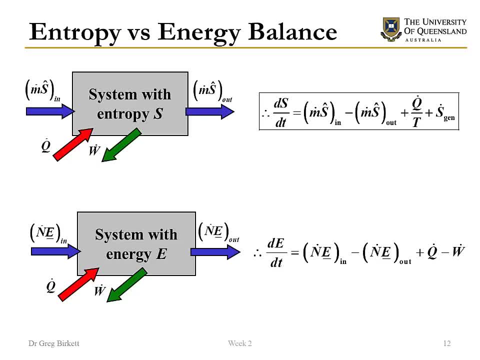 thing. then I can look at the entropy balance of the system And I'm going to contrast it here with the energy balance of the system. So with the energy balance, which is a conserved quantity, then we don't have any energy generation term. It's impossible. But with the entropy, 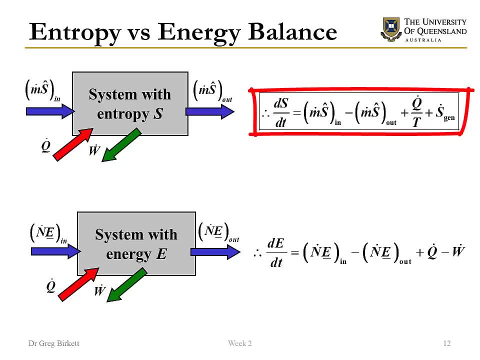 there are two or three key differences. We can still have an entropy balance. We can say that the entropy is changing with time. We can still have entropy coming in and entropy coming out of the system, But the heat term is divided by temperature, as per the definition of entropy. 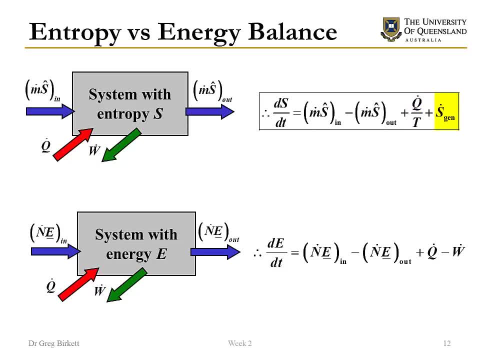 We have a generation term, which we don't have for energy, And then there's no work term for the entropy because we can't relate work directly with entropy. So these are the key similarities and differences between the entropy and the energy balance equations. 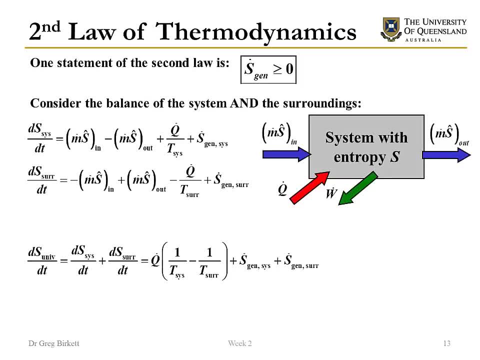 Now, if we look at the entropy balance, then not only can we do an entropy balance on the system, but we can do an entropy balance on the universe as well. okay, and so, and that's what I've got in these two equations here. now, if I add those two things together, then my mass flow, that's leaving. 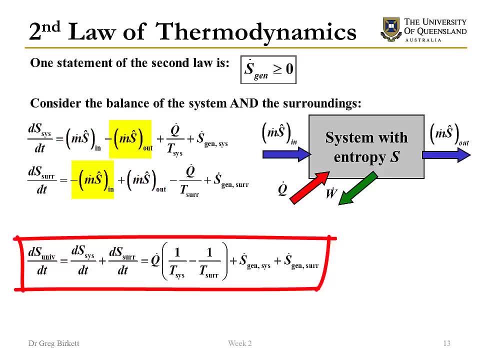 the surroundings and entering the system and my mass flow that's coming out of the system and entering the surroundings. those two things just cancel each other out and what we're left with is this temperature term down the bottom for the heat and then a generation term for the system. 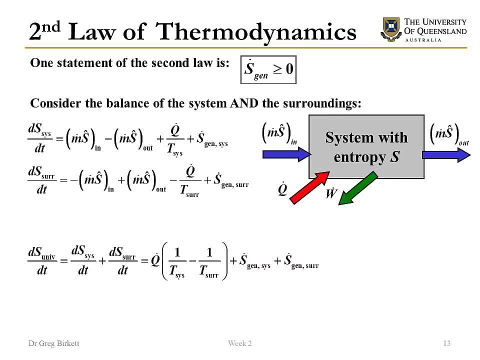 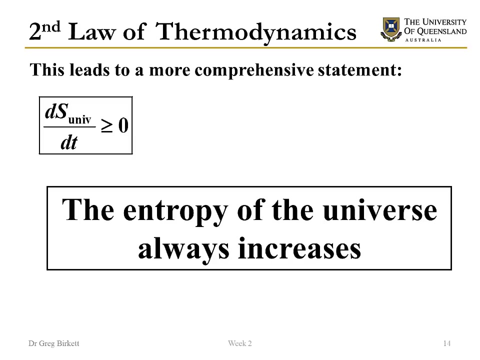 and a generation term for the surroundings. all these three terms must be positive, and so, as a result of that, then, the entropy change of the universe always has to be positive, and so this is the succinct definition of the second law, or of thermodynamics, and that is that the entropy of the universe always increases. 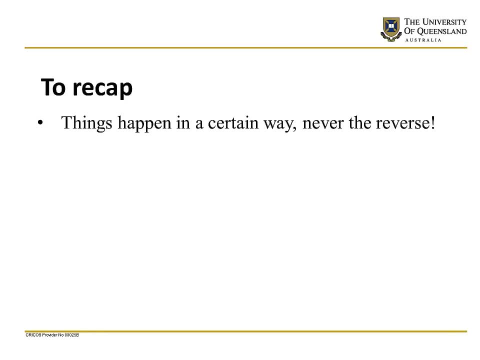 So, to recap what we've done in this lesson, Things happen in a certain way and never the reverse. Entropy quantifies this tendency, So this is why entropy exists as a concept and why we use it. Entropy is not a conserved quantity, and closed systems can generate entropy. 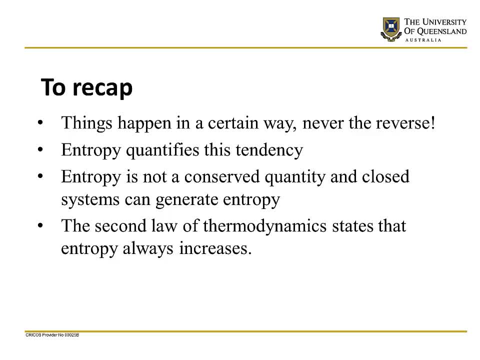 The second law of thermodynamics states that entropy always increases. Thanks for your time. 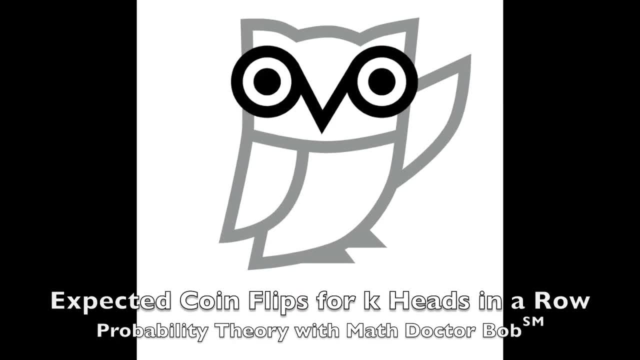 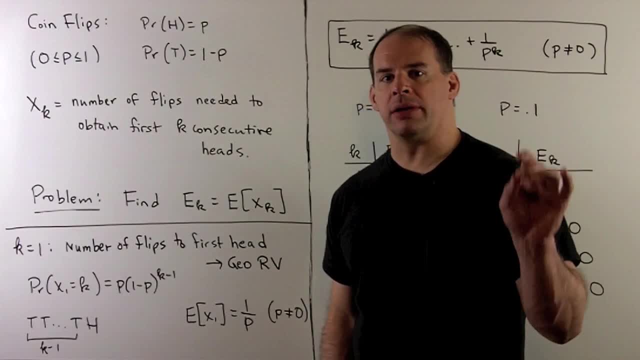 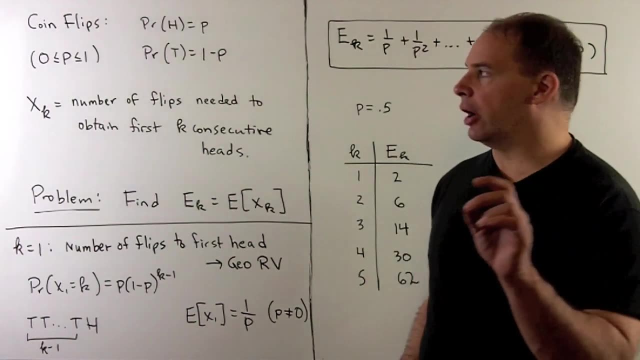 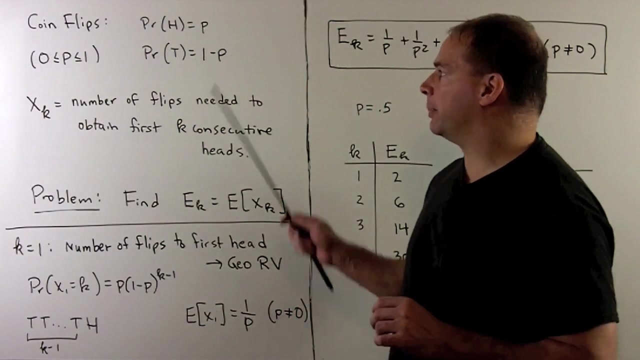 Here's an application of the conditional expectation formula with geometric random variables. Our scenario: we start by considering sequences of coin flips. For a coin, the probability of heads is going to be equal to p. where p is between 0 and 1 inclusive, Then the probability 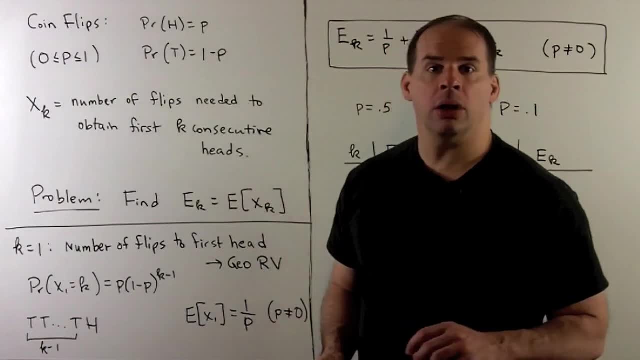 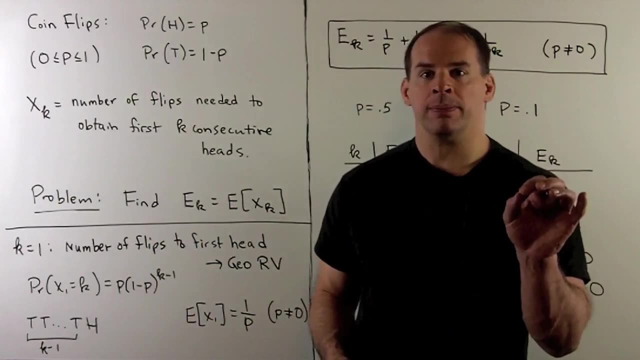 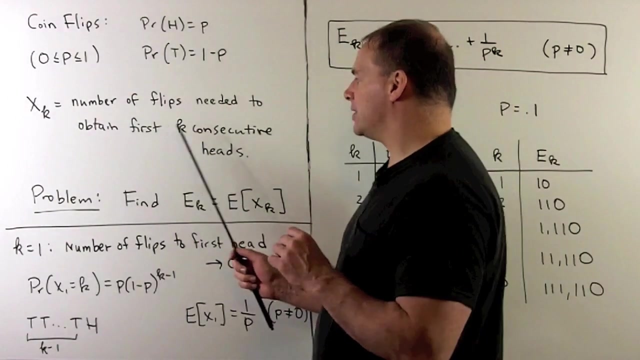 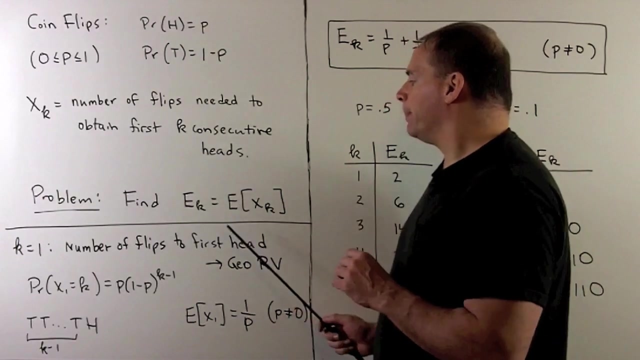 of tails is 1 minus p. We consider the random variable x sub k. So x sub k is going to take one of our sequences. It will return the number of flips that it takes to obtain the first run of k consecutive heads. Our problem: I want to find e sub k, the expected value of x sub k. So e sub k is just going. 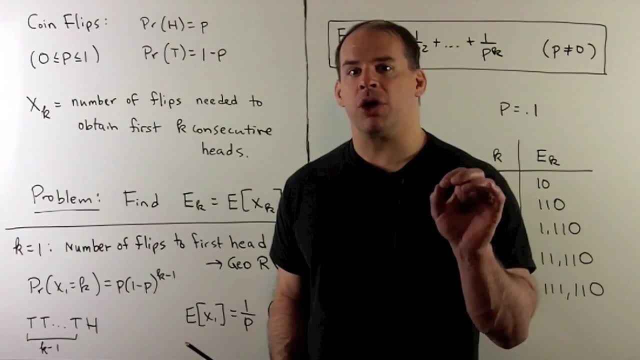 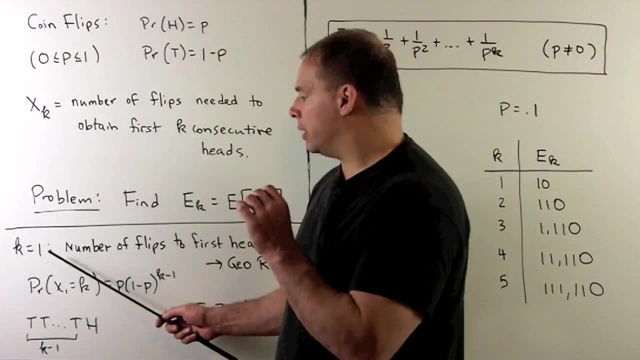 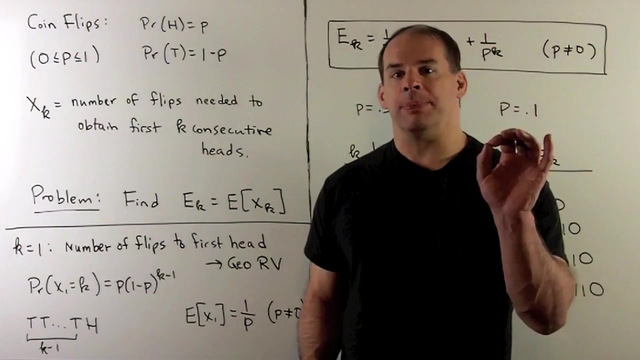 to be the average number of flips that it takes to get to our first run of k heads in a row. Now, when k is equal to 1, we're just trying to find the number of flips to get to the first head. That's familiar. That's going to be a geometric random variable. 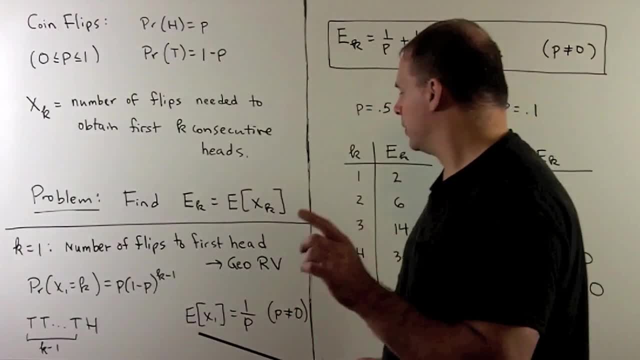 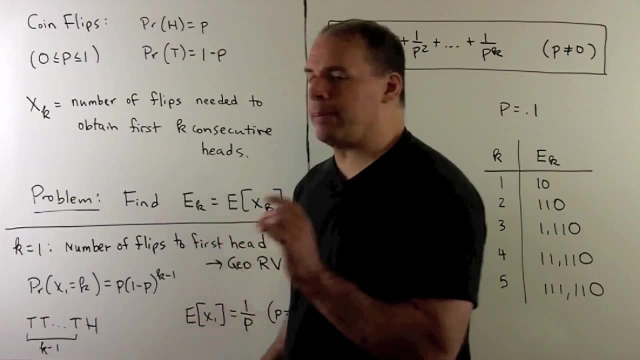 So let's note, if I want to know the probability, that x sub 1 is equal to k. well, if x sub 1 is equal to k, that means we have our first head occurring on the kth flip. So that means: